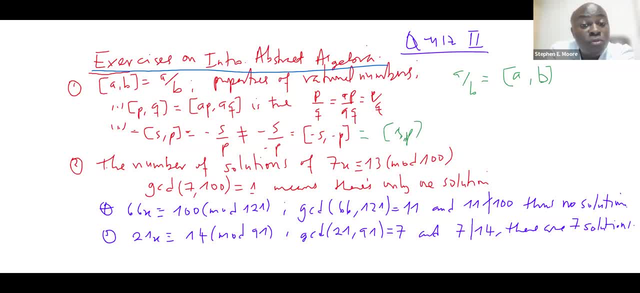 questions, And the other question was to find the number of solutions of a linear congruence And this. there are many ways to solve this, but a quick way of solving or going about the is a clear-cut understanding of the greatest common divisor, using the greatest common divisor. 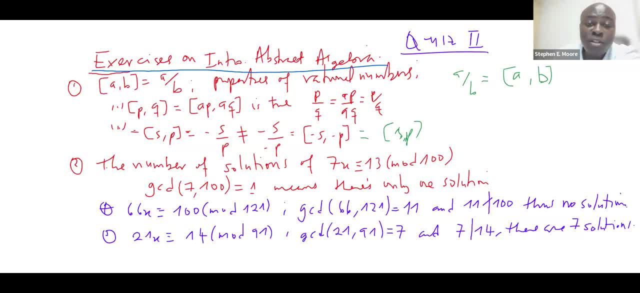 so if you are giving, if you are giving the number of solutions for 7x uh modulus uh is equal to 13 modulus standard uh. that what you need to do is you take the number here, seven, the gcd of the number here and the modulus. so if you take the gcd of seven and hundred is equal to one uh we. 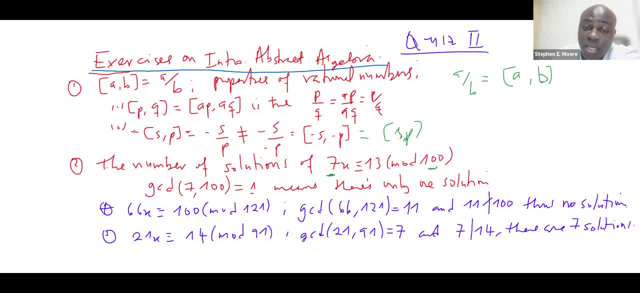 know that the seven, the gcd of seven and hundred is one and that means that there's only one solution to this problem. okay, so some examples are: if you are giving 66 of x- uh is equal to 100 modulus one, two, one, then you find the modulus, you find the gcd of 66. 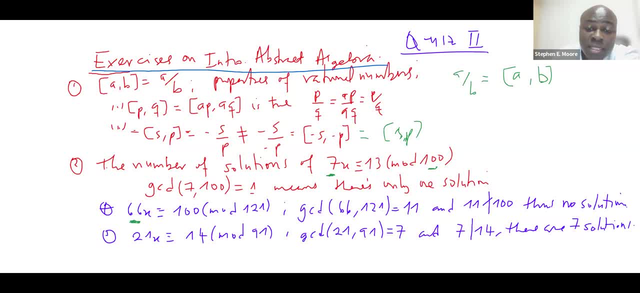 and and one through one, and then if you realize that the gcd of 66 and one to one is 11, and now you check if um this gcd right, this gcd divides um your hundred right here, in this case this hundred here, if it divides, then you know that there are a certain number of solutions. but if it, 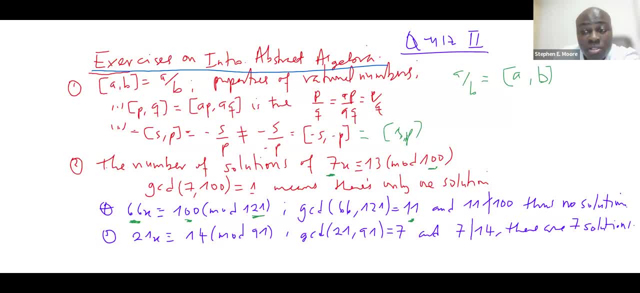 does not. then you say that there are no solutions. right, so there are no solutions because the gcd does not divide this 100 uh, that we have it. so another example is: if you have 21 of x, uh is equal to 14 modular 91. the gcd of this 21, right of 21 here, and and then 91, the gcd is 7.. then we say that the gcd is 21. So that means that the- if you can see that they are not divided away from 0 and the gcd is 21, which makes the 41 is equal to the blog going forward. so 9 & 21, if you want to get this. think of 21 before writing these up. that is, boundaries like a 0 if you write the gcd of 21 and you might have no way that you can write the descripcion to game. so the gcd does not divide conservatencally. so the that is not 1. that is the values that we have to write around the base of our terms to avoid our terms. so another example: 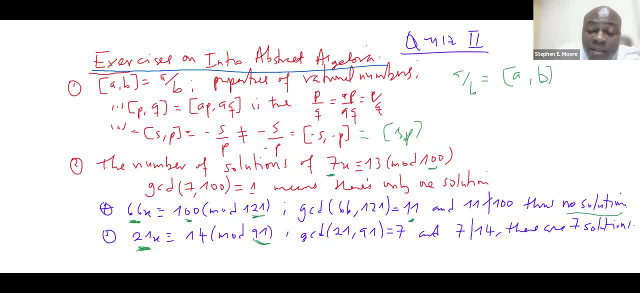 then we say that this gcd7 here divides right divides. so this gcd7 here divides 14. this 14 comes from here, right, and because it divides 14, we say that there are existing solutions to to this linear congruence. so this is a way to determine if there are solutions or how many. 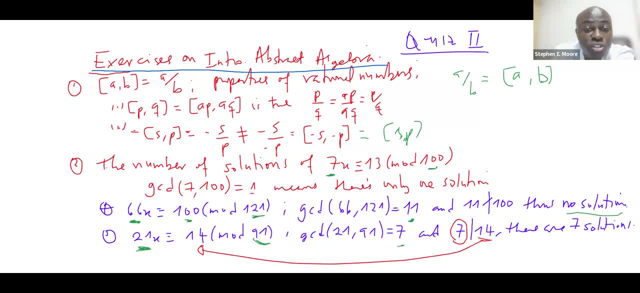 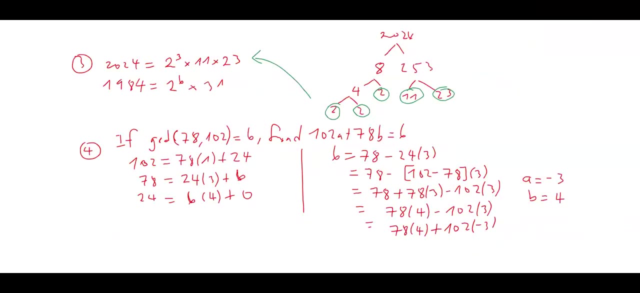 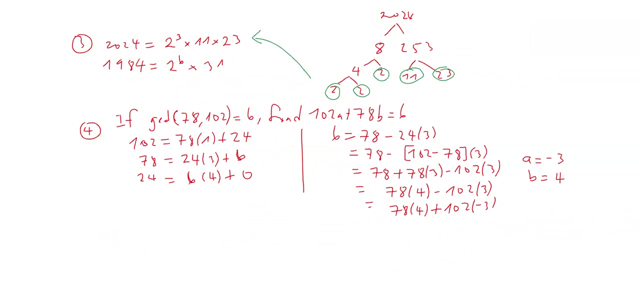 solutions there exist or there are no solutions to a certain linear congruence. okay, um, then we go to um finding, uh, in this case, you want to find, you want to find the, the factorization, uh, the factorization of 2024, 2024 and 1984, of course, um, just if you want to find the factorization of twin, something like a number, 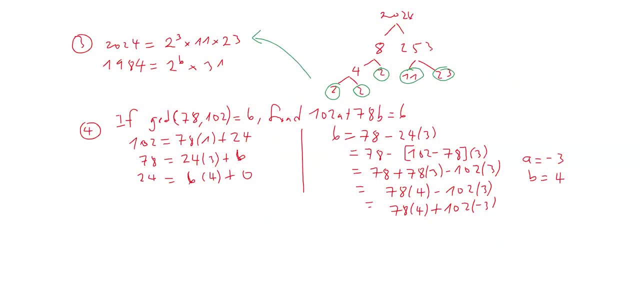 2024? um, you have to really look for the prime factors of that number, and the way to do it is: uh, popularly, what we used to do when we were in primary schools is something called, like, the factor tree, but the factor tree has limitations, so this, we just discussed it as well, so you try. 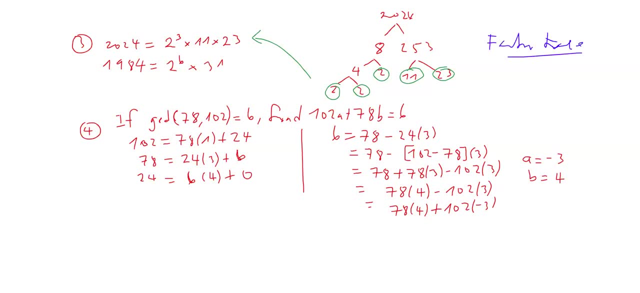 to to look for numbers that can divide, uh, this number. so there's, so you, you are left with only primes, right, only primes, primes only. if you are left in primes only, then you know that that is what gives you. so these two, uh is really- um, it wasn't really complicated- one uh. then we also spoke about 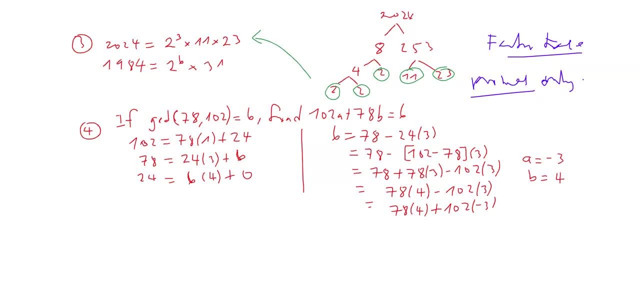 finding if you are giving that, if you are giving the gcd of two numbers. here we have 78 and 106, 102, the gcd is six. and then we are asked to find a linear combinations of 102 times a plus 78 times b, which gives you six, and to find this a and b. okay, so what we said was here. you cannot find this. 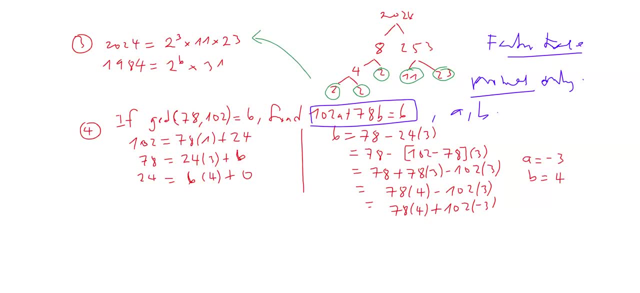 euclidean algorithm. you have 102 and 78. you can write 102 and 78 times 1 plus 24. then now you come 78. you take your 24 and then now you write your 78 to be equal to 24 times a certain factor plus. 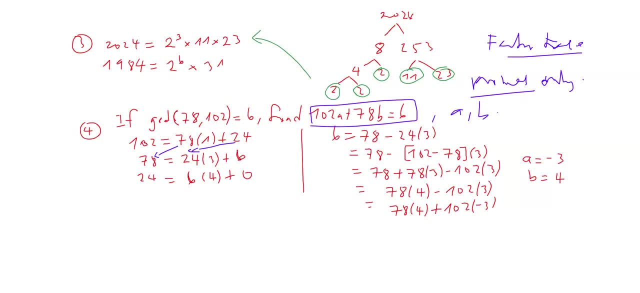 a certain factor. this is 24 times 3 plus 6, and now you take your 24, you take your 6, then you say that 24 is also 6 times 4 plus 0. so once you reach this part where this is 0, then you know that, uh, your gcd of 102 and 78, you really write a 6 as 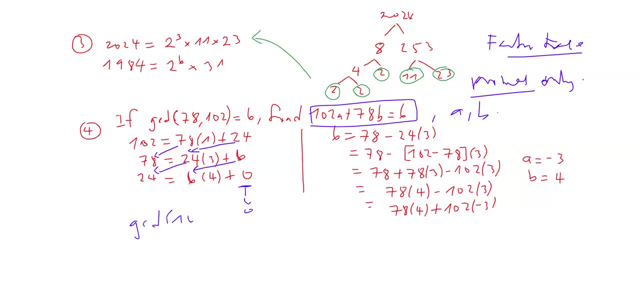 this one here, okay, and now what we want to do is we want to write, uh, this gcd, which is six, uh, as a linear combination of this, 102 and 78 times some scalers. so we start with six and then we- we usually start with the lot, but one line here, right, we usually start with this line. 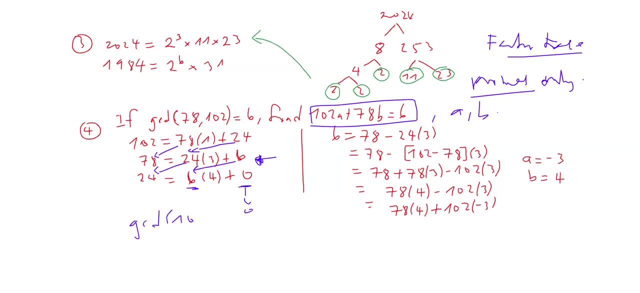 here where we start from. then we say that you can write six, the gcd6. you can write it at 78 minus 24 times three and then you're 24, you're 24. now we go to the 24 of the linear combinations. then we write it at: 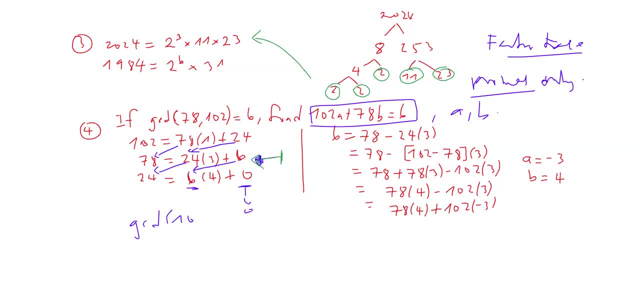 Now we go to the second line. We can write 24 as a combination of 1,, 0,, 2, and 78. So we replace 24 now by this combination and then the 3 still remains. If we do that now, we can multiply through and factor out. 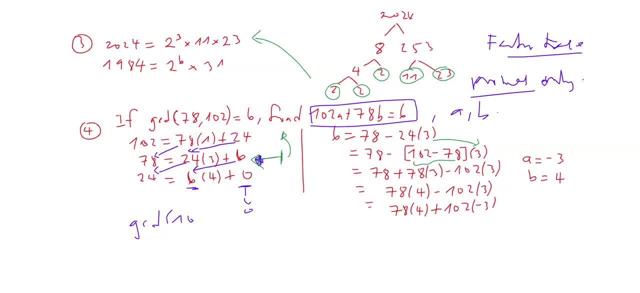 We do this, We have 78 times 4 plus 1, 0, 2 times minus 3.. And this gives us what we are looking for. 1, 0, 2 times A plus 78 times B should give us 6.. 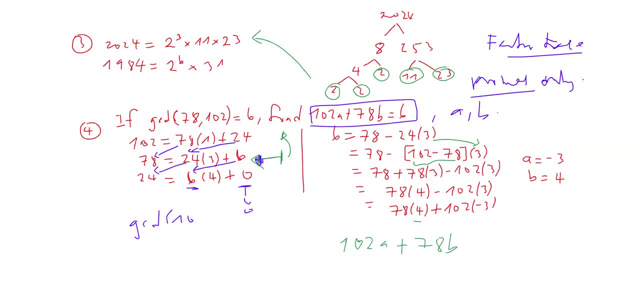 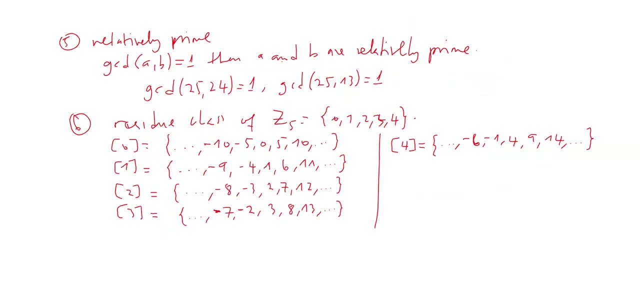 So we're able to now determine this A and B in such a manner. Next we ask the question of relatively prime numbers, And I've opposite. the definition Relatively prime means that a GCD of 1.. So if two numbers are relatively prime, then their GCD is 1.. 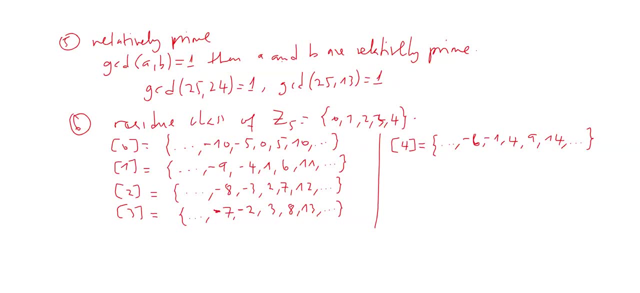 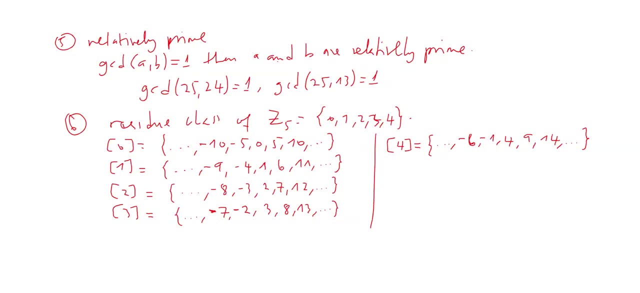 So if we are asked to find a relatively prime number of 25, then you need to look for the numbers such that the GCD of those two numbers gives you a 1. And so here we're leaving 25.. So we look for all the numbers such that they give you this. 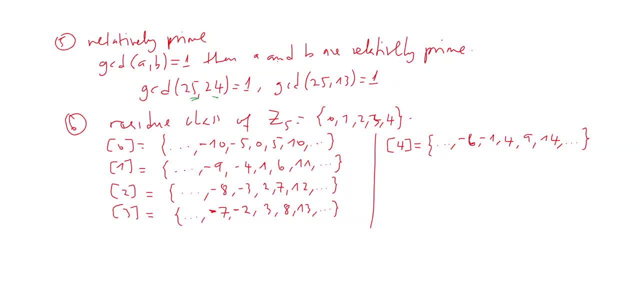 Together, 25 gives you 25.. And the next question was to ask we were asked to solve was to find the residue class of modulo 5.. So if you know how to find the residue class of modulo 5, you know that, simply, if you have 0,, if you have 0,, 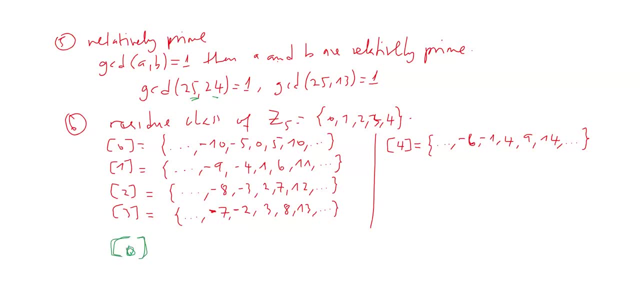 then you need to find the GCD of 1.. So if you find all the entries here such that they can divide, it is divisible by 5, or it is divisible by 5, and then you get an integer okay. 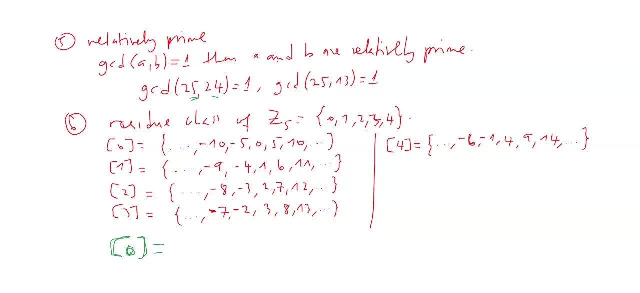 You get an integer or you get a residue in that manner as well. All right, so we said that if you have this residue class, it just means you have n minus some 0 over 5.. And then now we know that it should be an integer. 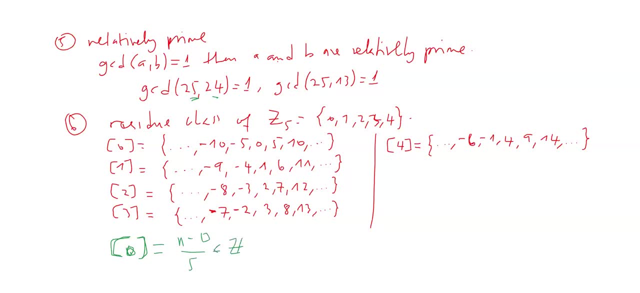 So we need to find all such n right, Find all such n which are also integers. So, for instance, if we take this, we take the 0, that residue 0, residue class 0, we know that if n is minus n, 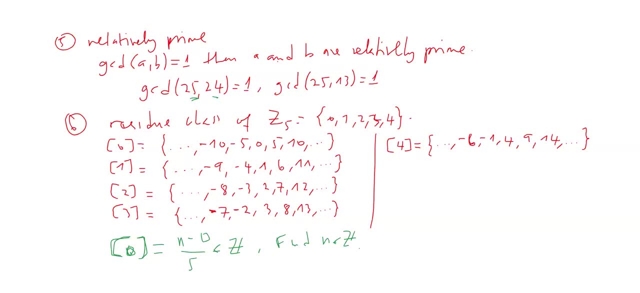 so, for instance, here we can have minus 5, minus 0 over 5.. So this is equal to minus 5, and this, if we go to minus 1, right, it's equal to minus 1, and this is an integer as well. 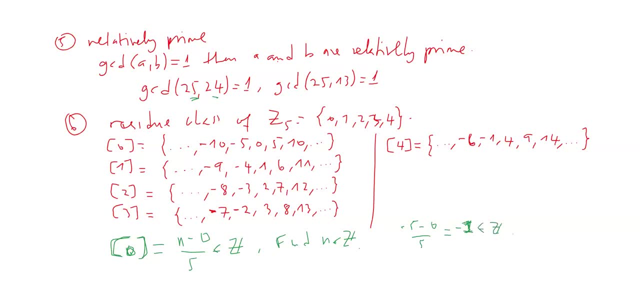 So we look for only integers and in that sense we're able to create the residue class. So for 0, we can write it for 1, we can write n minus 1 over 5 to be integer. 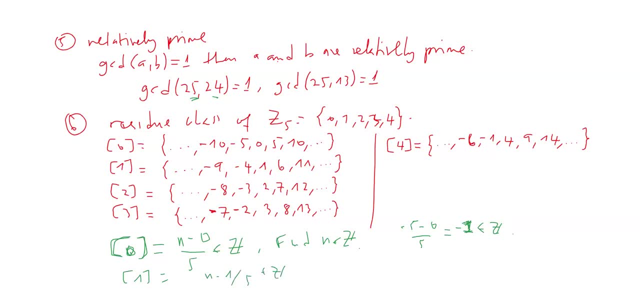 So we need to look for integers. All the entries n find that n minus 1 over 5 will still give us integers. If we come here, you see we have, for instance, here we have 1.. You understand that if you have 1 minus 1 over 5,. 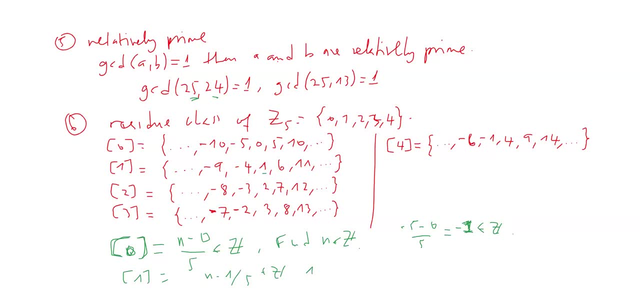 this is 0, and this is an integer. That is why 1 is here. okay, and so on. So if we do that, because we are in module 5, we know that we need residue class 0, residue class 1, up to residue class 4, okay. 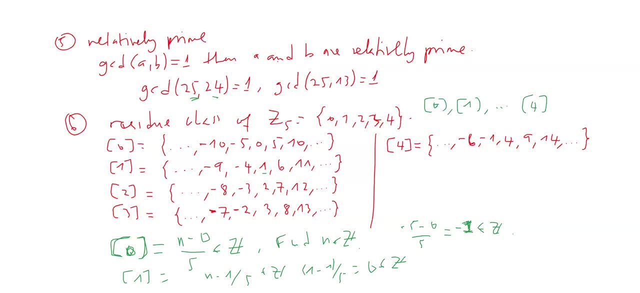 And then you shouldn't forget what we said about some properties of the residue class. We, when we spoke about the residue class, we said the residue class creates partition and the union of all the residue classes, okay, will give us, will give us the whole set. 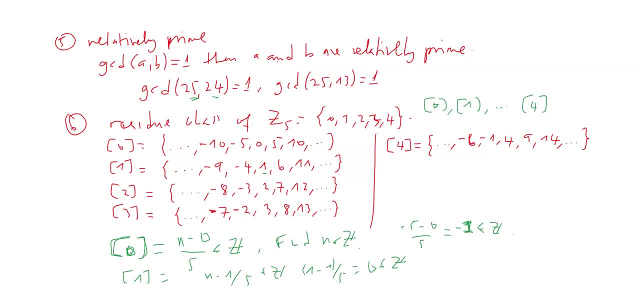 So these are properties you shouldn't also forget. And so you will see that, Okay, So we have the whole set. Okay, So we have the whole set. So you will see that if we take, for instance, this residue class, 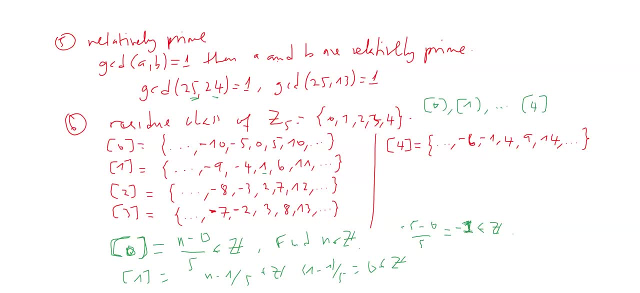 in this case we can see that we can create the whole set Z if we just take the residue class 0,, union 1, union 2, up to union 4. It will create the whole set Z, normal system Z for us okay. 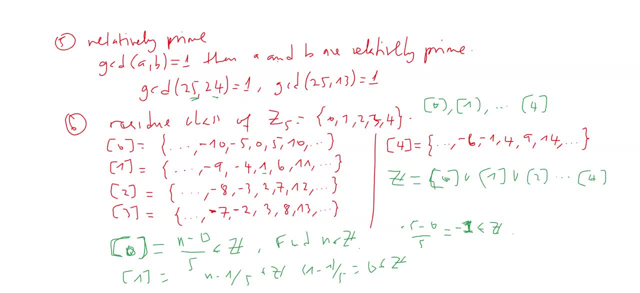 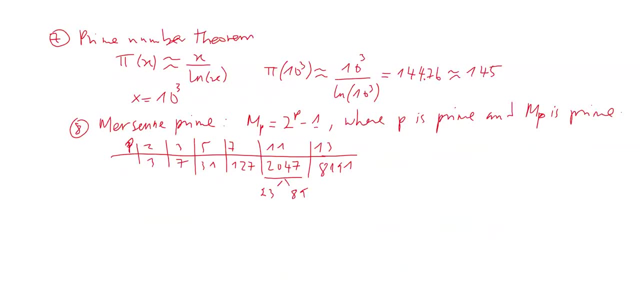 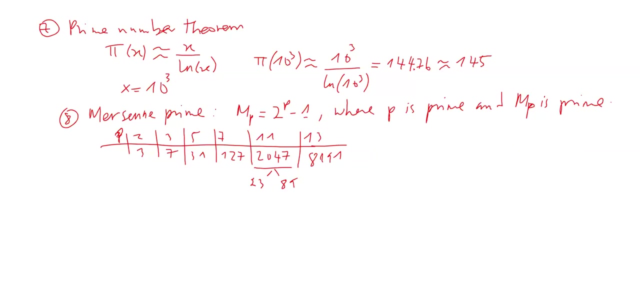 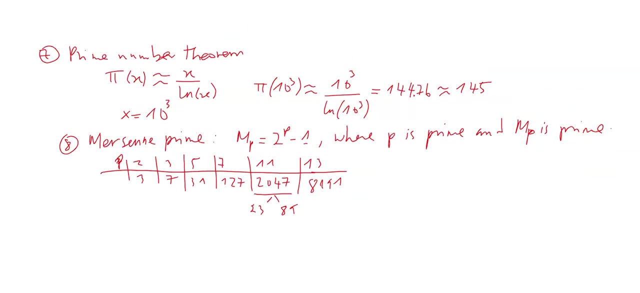 Okay, Then next. Next, we did ask questions on prime number theorem. okay, prime number theorem. So just to give a formula for prime number theorem, this is the formula for prime number theorem. So for prime number theorem, we get your formula and we say that if you write: pi of X is approximately equal. 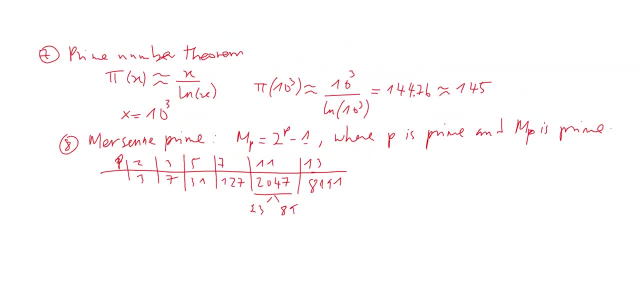 to X over length X, And that is the prime number theorem. So here we chose X to be 10 to the power 3.. So this is: pi of 10 to the power 3 is approximately 10 to the power 3 over length 10 to the power 3.. 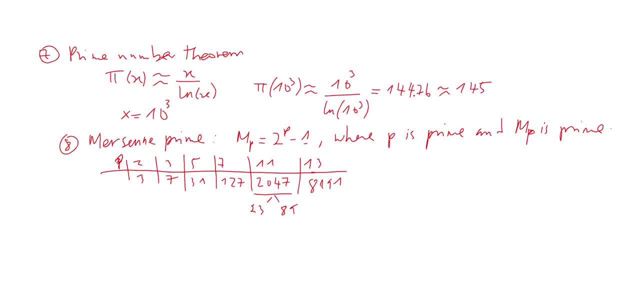 And this is equal to 144.7,, which is approximately 145.. So it doesn't matter if I give you X to be 2 times 10 to the power 3.. All you have to do is you find times 10 to the power 3, right is approximately 2 times 10 to the power 3, over length of 2 times 10 to the power 3.. 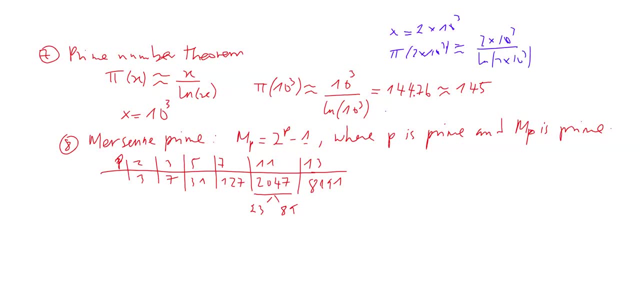 So this is how you find these numbers. Of course, usually I approximate them, I round them up. So okay, then the next one was the messing prime. So we said that the messing prime is a prime number which is following such a formula: MP is equal to 2, to the power P minus 1,. 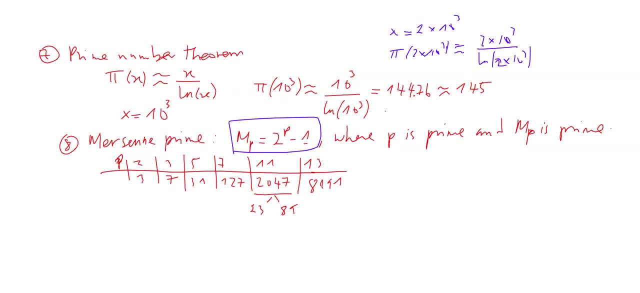 where P is prime and MP will also be prime. So if P is prime and MP is also prime and we say that this MP is a messing prime, So it's not really a tricky question, but it's just an understanding of what this means. 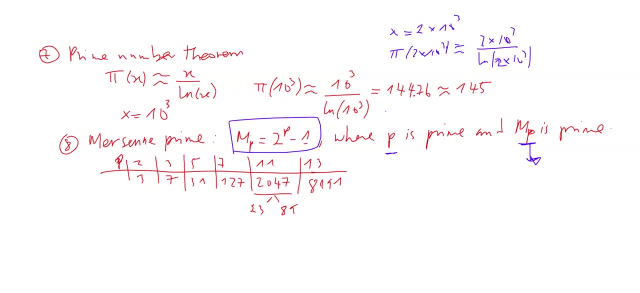 So here. So here you see that if we take for instance all the prime numbers 2,, 3,, 5,, 7,, 11,, 13, if we take, use the same formula here, MP is equal to 2, to the power P minus 1.. 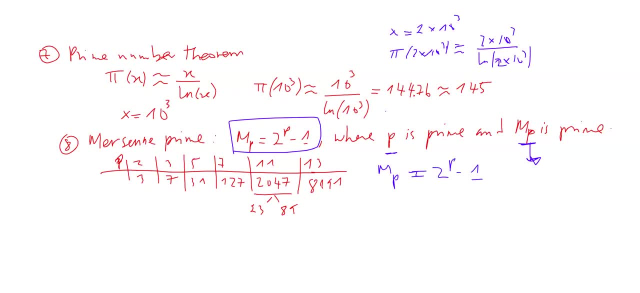 If we take P to be 2,, we'll get 3, and 3 is also a prime number, So we say that 3 is also a messing prime. Okay, If we take 3, which is a prime number, 3, we'll get. 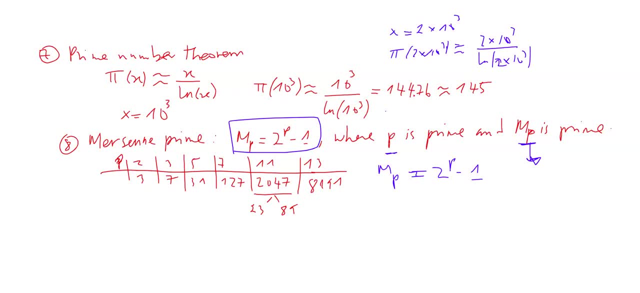 Here. Okay, We'll get here. We'll get 7, and 7 is also a prime number, So it's a messing prime. It follows the formula 2 to the power P minus 1, and then, if we take 5, we'll have 31.. 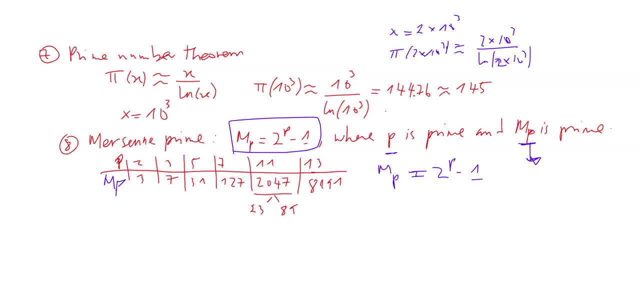 So 31 is a prime number and 5 is a prime number, So we have a messing prime 31.. If we take 7, we have 127.. This is a prime number. So we say that it is a messing prime. 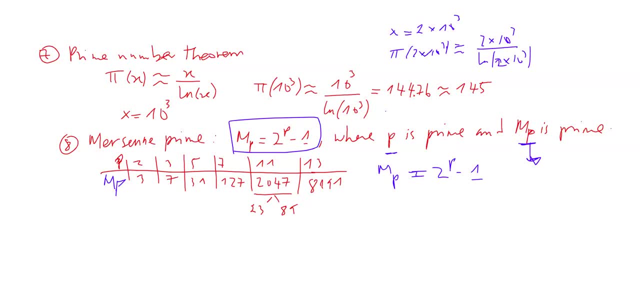 It follows the formula. But if we take 11, we will see that 11, if we put P, is equal to 11 in this formula, we'll get 2047. And we realize that 2047 is not a prime number. 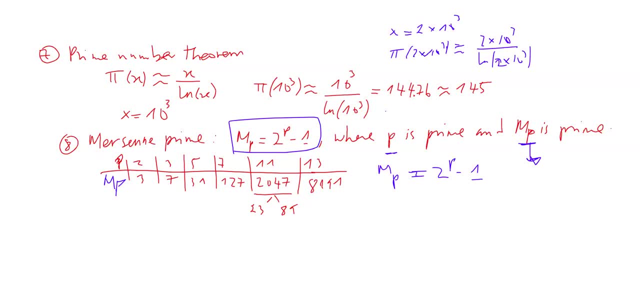 So 2047, right is equal to 23 times 89. So it is not a prime number, right? So in that case, although So this is a prime number P, the resultant here, which is 2047, is not a prime number. 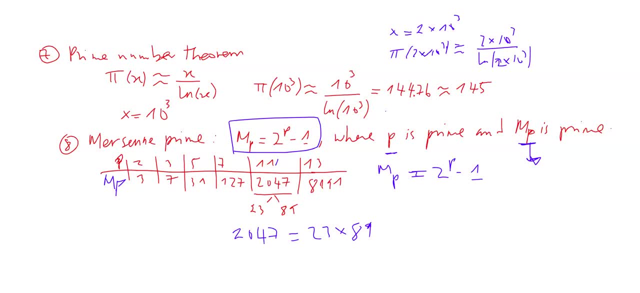 So it is not a messing prime. So this one is not, does not qualify right. It's not because it is not a prime number. So there are many numbers you can generate from this, using P to be prime, but not all of them will end up giving you NP, which is also a prime number. 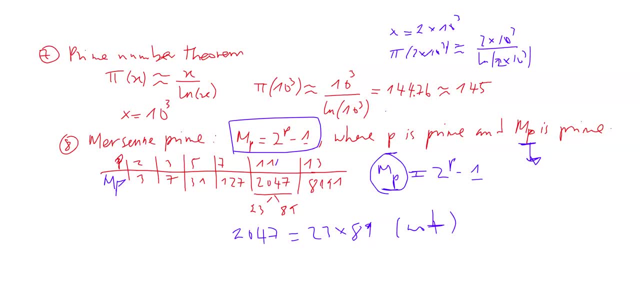 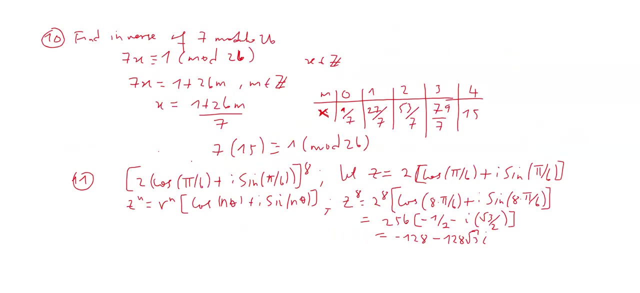 Those, Those ones which end up with NP also as prime number. We call that a messing prime. Okay, So then the next one was to find the inverse of 7 modulus 26.. So you can write such a you can. you can write such a statement, as 7x is equal to 1 in modulus 26.. 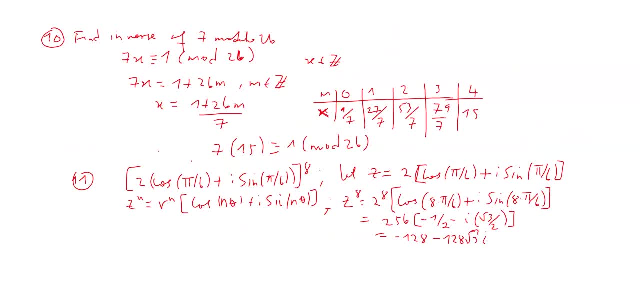 And this: you can write it As: 7x is equal to 1 plus 26 M, When now your x is equal to 1 plus 26 and over 7.. So if you do that, you, and then you take M for every M, you can do it for every M. 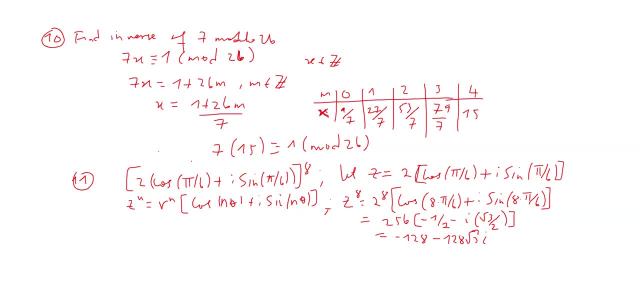 You can check what x will be right. So here, of course, you shouldn't forget, We are looking for x, Set that x. We are looking for x, Set that x. It's also an integer. Okay, so that x is also an integer. 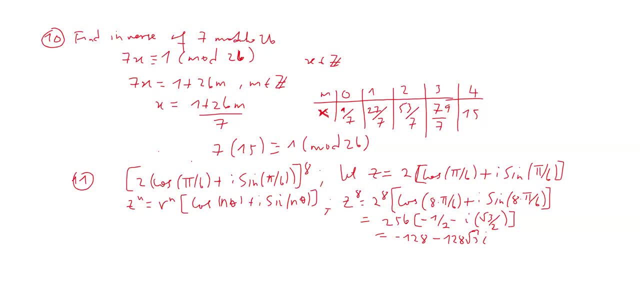 So here we draw a table: We put M to be 0. Then we calculate for x: We get 1 over 7.. We put M to be 1. We get 27 over 7, and so on until we put M to be 4, and then immediately we get 15.. 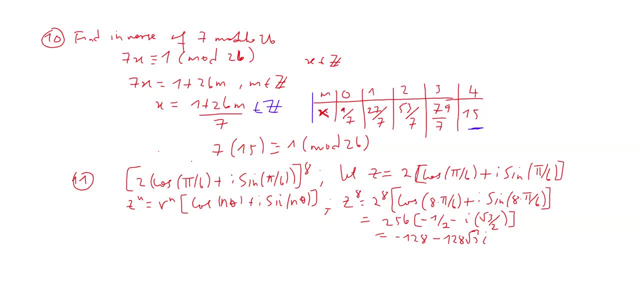 So in that sense we say that If we take, if we put 4 here, we'll get 15.. And so 15 will be the inverse of 7 in modulo 26.. And the next one was to find, was to was something in the sense of complex numbers, of nth. 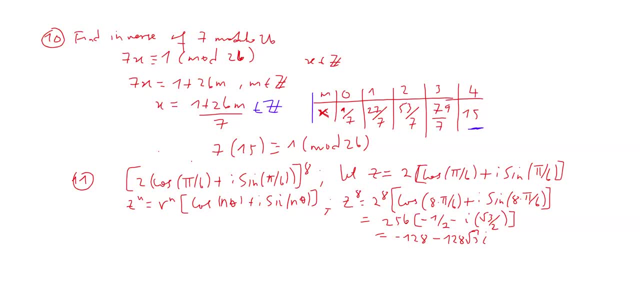 Okay, of nth order. So we're giving true cause Pi over 6 plus i sine pi over 6, all to the power 8.. And we're told to find the complex values in the complex domain coordinate system Right Complex coordinates. 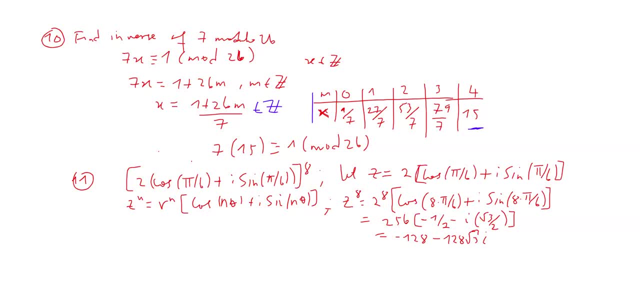 So we use the formula that we know that if we want to find at the 10th root, then we know the nth power, then we know our n is equal to 4.. So we're subtraining and finding nth per eta. 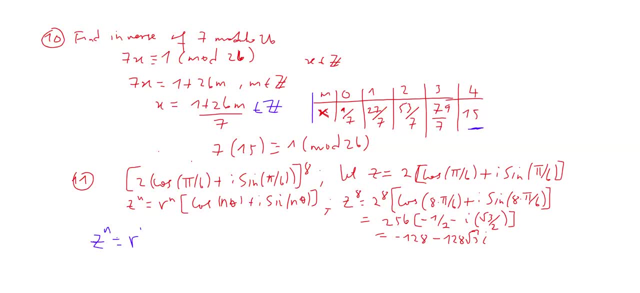 So that's nth is equal to 5 pi. 5 pi r times 5 plus i sine nth. Because of this, we're ordered with this Informationen, And so thisife is one orden, But we have this logged out element. For this we've got the parameter nth, which is 획 and theta plus i and theta. So what are we gonna do next? We're gonna club by symbol here and then literate this- okay, Because for simple numbers we're gonnaitions- just to undefine it as nth, but with nth. Here. what's this here? There's a play here, The k betrayal here. The k demands here and v zero is v 0,. okay, V 0, correct. So we get 21 over 7, plus i nth. 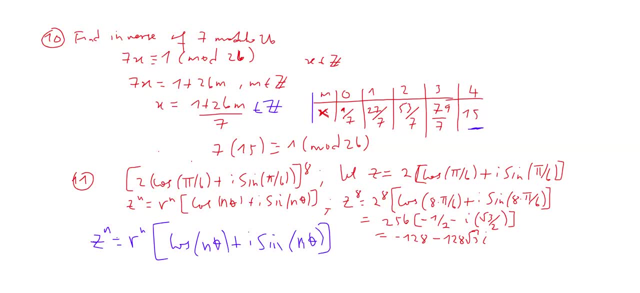 Okay, plus sine n theta: Okay. so in that sense, if we write here, then what we do is that we know that we are dealing with n is equal to a, And then our theta is 5 over 6.. So we can rewrite now our equation in terms of this formula here: 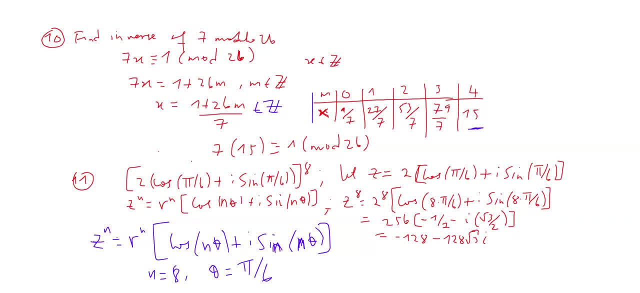 So z of 8 is nothing but 2 to the power. 8 cos 8 times. now the theta here is pi over 6, plus i sine 8 times the theta, which is pi over 6.. 8 to the power, 2 to the power 8 is 256. 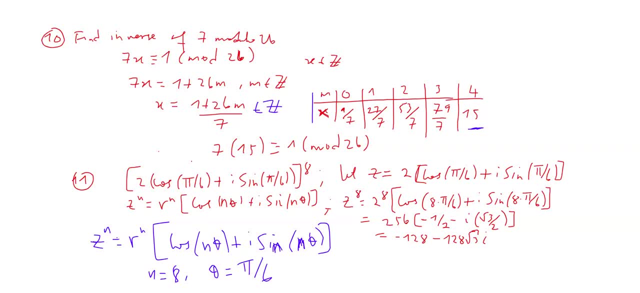 Then now cos 8 times pi over 6,, which is 0. So this, which is like 240 degrees, happens here in this bracket where it is minus x and minus y. Okay, you come here, and then this is 8 pi over 6.. 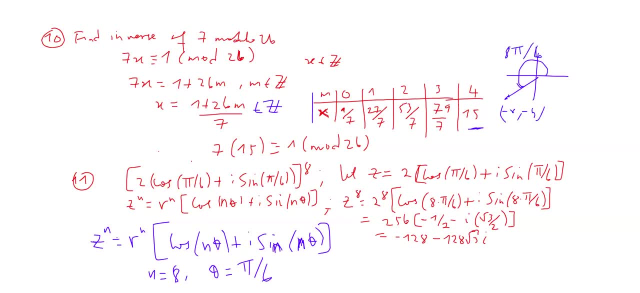 Okay, 8 pi over 6.. So if you do that, then you know that you have a 60 degree angle here, 5 over here. you have a 60 degree angle here. that gives us minus half, And then of course as well on the sine direction, it gives us minus square root of 3 over 2.. 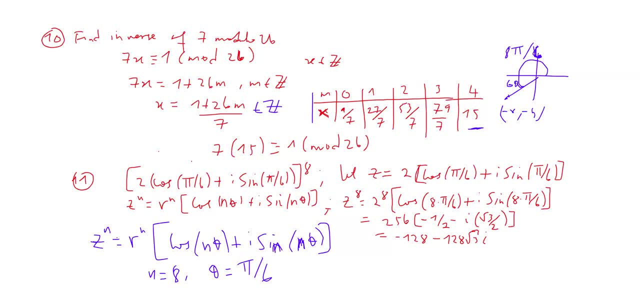 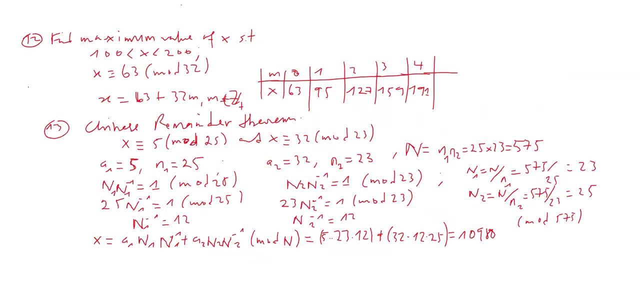 So if you multiply through then you have minus 1 to 8, minus 1 to 8, square root of 3 of i. Okay, complex. The next question is to find the multiple value of x. x is between 100 and 200.. 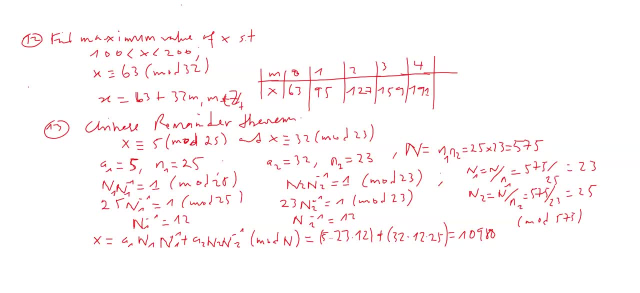 Can you define the linear for x to be equal to 63 in module 32?? For x is equal to 63 in module 32, I'll be writing as x. I'll be writing as x is equal to 63 plus 32.. 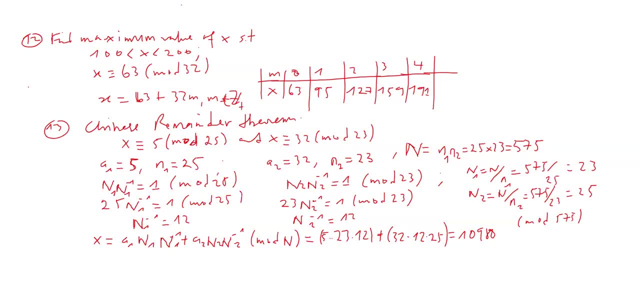 m, where m is an integer. So all we do is I draw a table of m and x. If I put m to be 0, I have 63,. if I put m to be 1, I have 95,. if I put m to be 2, I have 127,. if I put m to be 3, I have 159,. 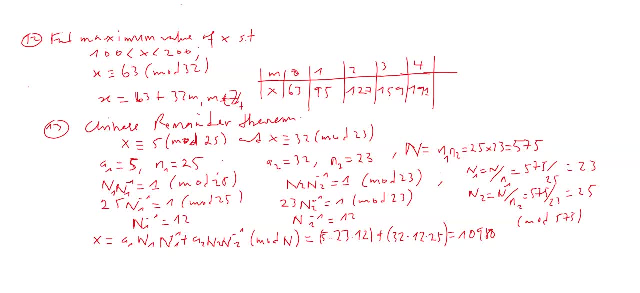 if I put m to be 4, I have 190, 1 of course, then it means that if I put m to be 5, I'm already out of bounds, because it is going to be 32 times 5 plus 63, and this is going to be 223.. 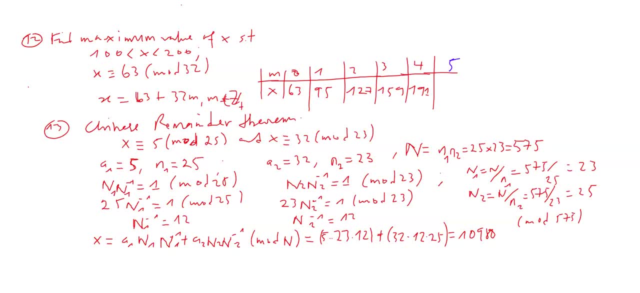 So I'm already out of bounds. So the maximum value for x is really 191 in this case. Then of course the next one was the Chinese remainder invariant application. here we are giving a question that X is equal to 5 in model 25 and x is equal to 32 model 23.. 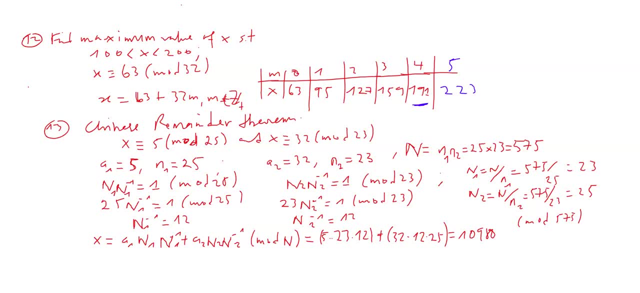 So what do you do here? we know: a1 is this value, here a1, and then a2 is this value, here 32, a1 is 5, a2 is 32.. And a1 is one, two, three, four, five, six, eight. a two is one, two, three, five, six, eight. a two is five, a two is thirty-two. 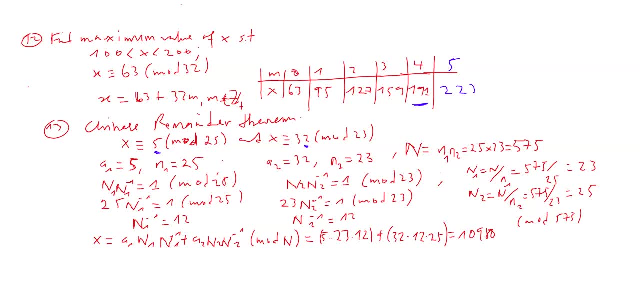 a two is thirty-two, N1 is this value here, which is 25, and N2 is this value here, 23.. Then we create a product of the modulus, So we call it a big N, which is now the modulus N1 and the modulus N2 multiplying together to give us 575.. 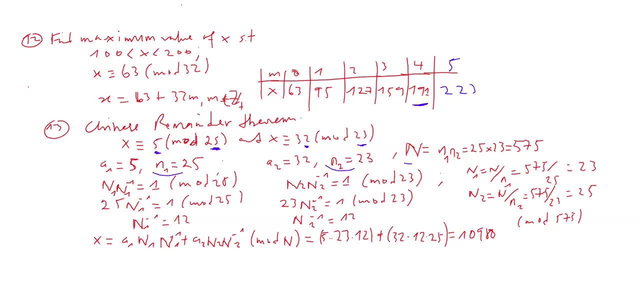 Then the next thing we do is that we calculate these volumes. here We calculate this: capital N1, capital N2.. So capital N1 is nothing but this big N over the small N1. That gives us the capital N1, which is here 23.. 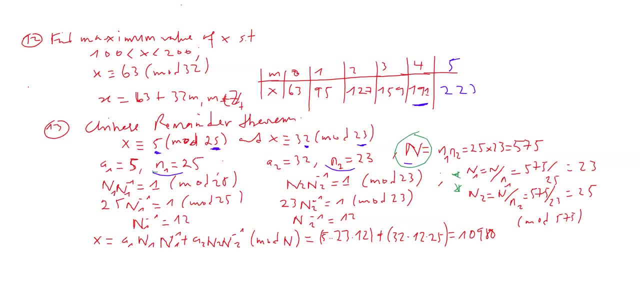 And then we do capital N2, which is now the big N, again over N2, the modulus N2. And then this is also 25.. And the next thing is, we calculate the multiplicative inverse of these modulus, So of modulus N1, the big N1, and then also of the big N2.. 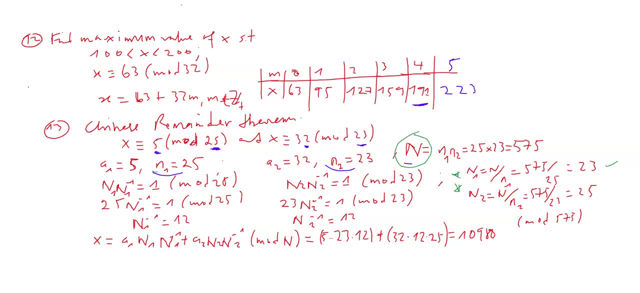 So if we have the N1, the big N1 is 23, right, And then the big N2 is, So we find the multiplicative inverse of N1, and then the multiplicative inverse of N2.. The big N1 and the big N2.. 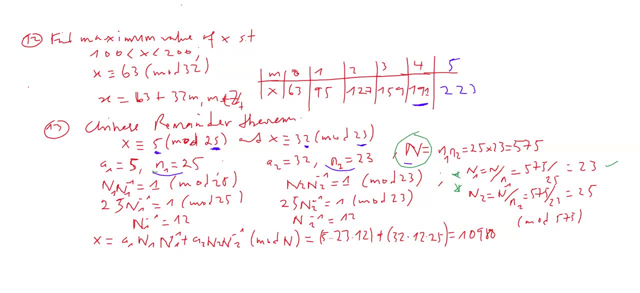 Capital N1, capital N2.. So to find the multiplicative inverse of N1 of 23,. N1 is 23.. Capital N1 is 23. Its multiplicative inverse is 12.. And then capital N2, which is 25.. 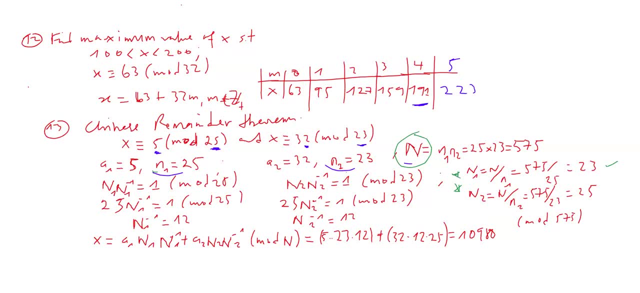 Its multiplicative inverse as well is 12.. So once we have that, then we can write now follow formula: A1, N1, A1 times N1 times the multiplicative inverse of N1, plus A2 times N2 times the multiplicative inverse of N2 in a big modulo N. 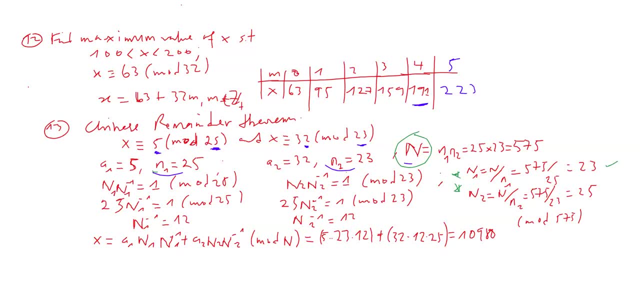 So if you follow that, then you will see that A1 here is 5,, N1 is 23, and multiplicative inverse of N1 is 12.. Plus here, so we have A2, A2 is 32,, N2 is 25, and its multiplicative inverse is 12.. 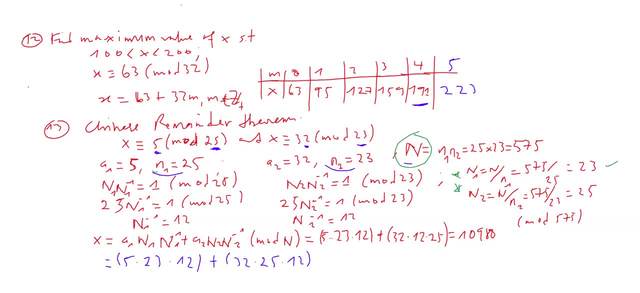 If we do that and we solve, We'll get 10,, 9,, 8.. And this, of course, will be in modulo 575.. So when we have this, so it means that we have. We have X is equal to 10,, 9,, 8, 8 modulo 575.. 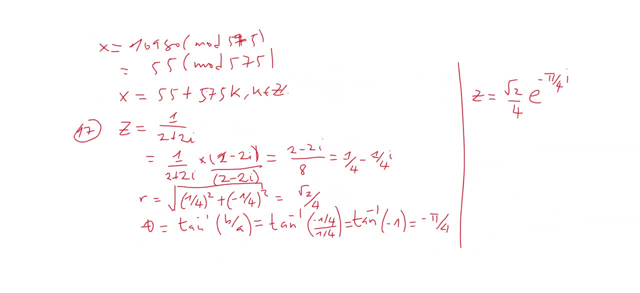 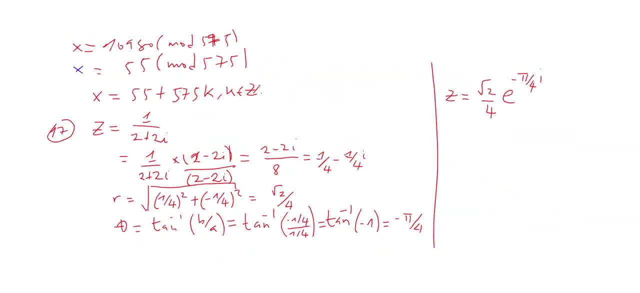 And this is the same. So we have X, and this is the same, as X is equal to 55 modulo 575. And this gives us- We can write it now as this- and then this gives us our final solution, Of course. 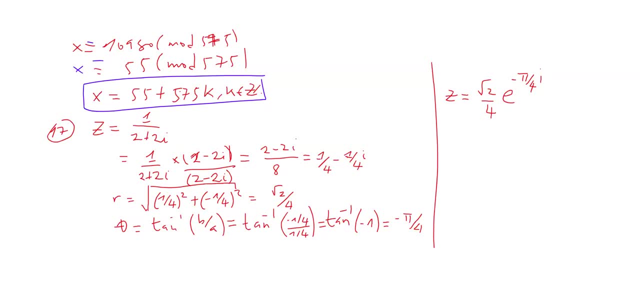 you'll be wondering: why is X equal to? Why is X 10, 9, 8, 9, 8 modulo 575, right The same as or equal to X 55 modulo 575.. It's really not a difficult thing, because if we 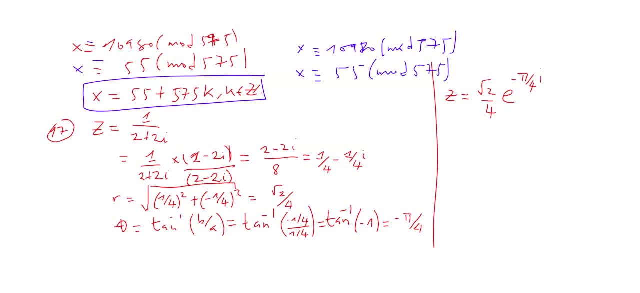 It's really not a difficult thing, because if we, If we take 10,, 9,, 8, and we divide by 575,, If we take 10,, 9,, 8, and we divide by 575,, we realize that there is a remainder of 55.. 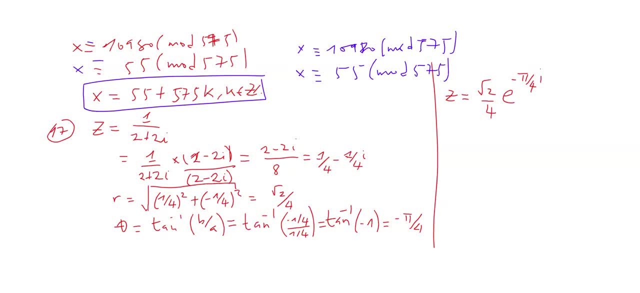 And that actually means that they are equivalent. You can write them as equal, or is the same, or is equal to. So we can write also this equation And that finally gives us the right result. Then next, we did talk about the complex numbers. 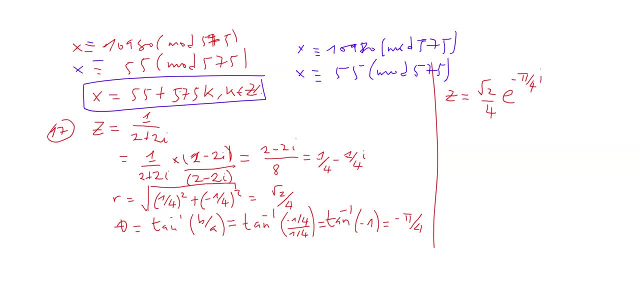 So here we are, given 1 over 2 plus 2i, And we are actually find or write it in an exponential form. In an exponential form. So for such a problem, what you do is, of course, you need to multiply this by the conjugate. 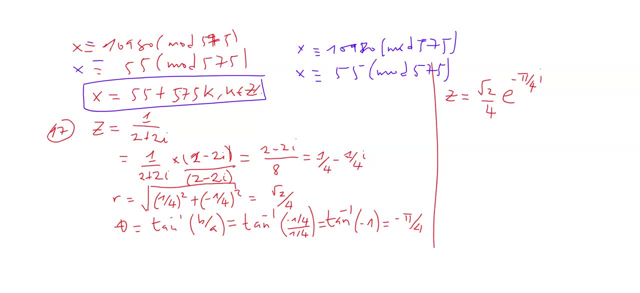 by the numerator and the denominator, the conjugate, And then if you do multiply by the conjugate, you multiply through, You multiply through. then you get 2 minus 2i over 8.. And this is equal to 1 over 4 minus 1 over 4i. 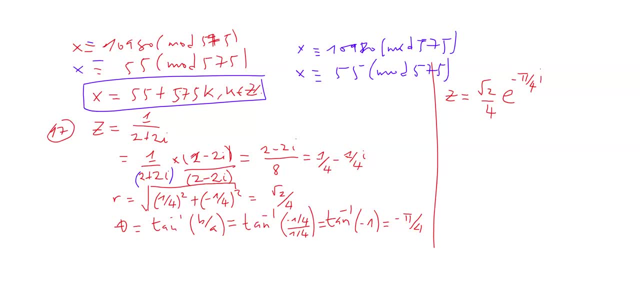 And once you have this, which is your x plus iy, now you can write the modulus, The modulus which is the square root of 1 over 4 squared, plus the square root of minus 1 over 4 squared, And this is square root of 2 over 4.. 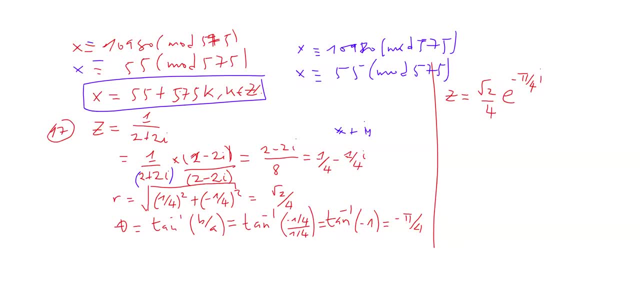 And now we can find the angle theta. The theta is nothing but the tan inverse of x over y, Or you can say it's y over x, Or you can say it's u over h. Whichever way you want to call it. 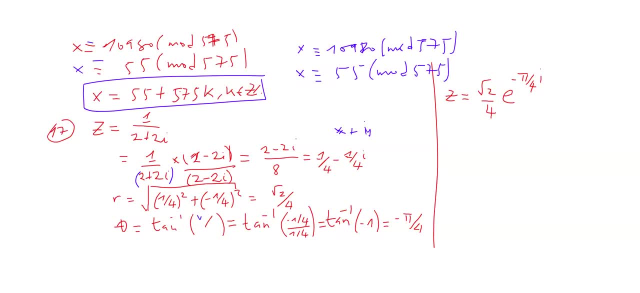 And this really means it's minus 1 over 4 over 1 over 4.. The tan inverse of that, And that gives us the tan inverse of minus 1, which is equal to minus pi over pi. And this now we can write our z in exponential form. 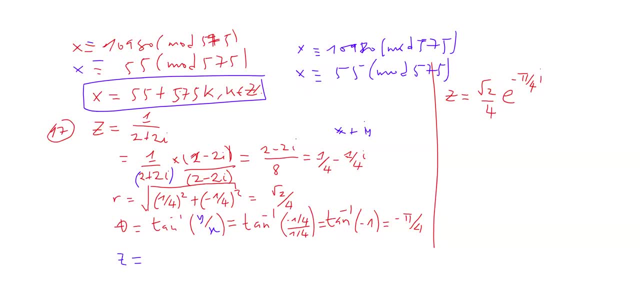 which usually looks like that, by theta of pi. So in our case our r is square root of 2 over 4.. And then our theta is minus pi over 4 over pi. So of course you can also write this in a polar form. 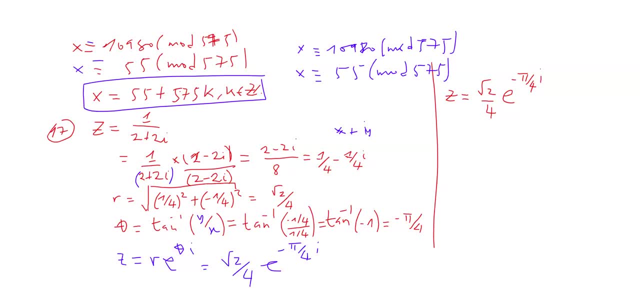 You can write it in a polar form, which is going to be that, And then you can have cos minus pi over 4, plus i sin minus pi over 4.. You can write it as well in a polar form. So one needs to understand how to go from polar to exponential. 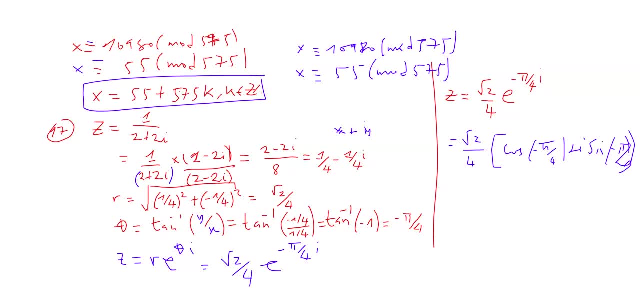 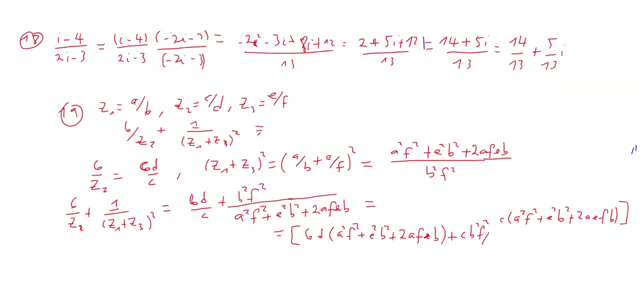 and then back course as well. Then the AT we're asked to find again to write this complex number, to compute the real and imaginary part of this complex number: i minus 4 over 2, i minus 3.. It's really not tricky. 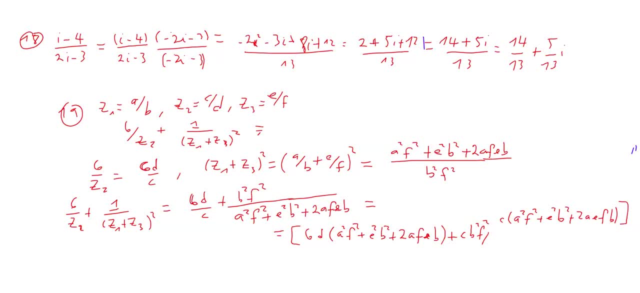 If you look at the denominator 2 i minus 3, you want to write a complex conjugate of this, So you need to be a bit careful And write this as minus 3 plus 2 i Right, Minus 3 plus 2 i. 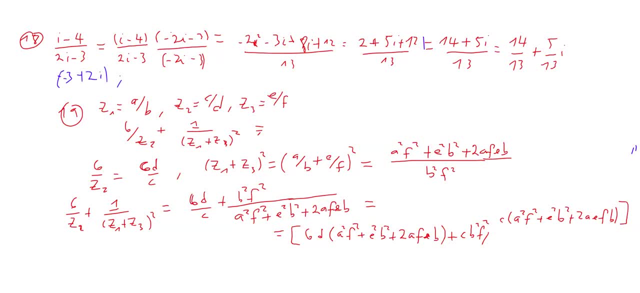 So that its conjugates, its conjugates now become minus 3, minus 2 i. Okay, So that's the only trick, only trick you need to use here to be able to get the right answer. So here you need to use this conjugate. 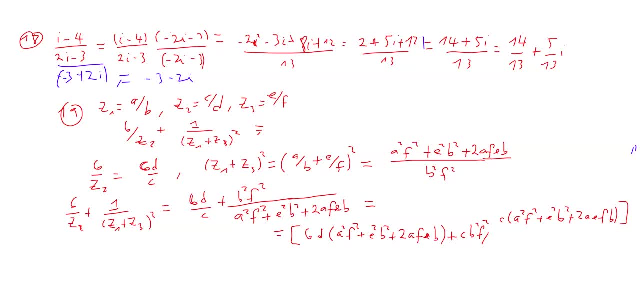 then you multiply it by the numerator and the denominator, You expand. So if you multiply here i minus 4 times minus 2, i minus 3.. If you multiply, you have i minus 2, i, which is minus 2, i squared. 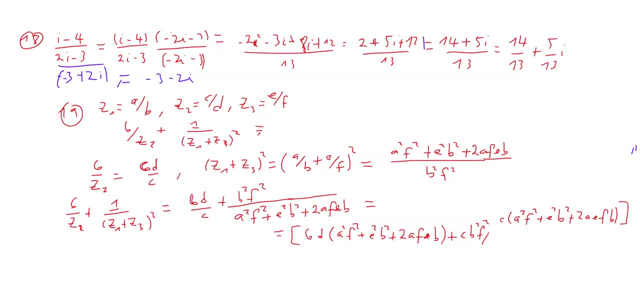 Then you have minus 3, i plus 8, i plus 12, all over 13.. Then this is equal to this: is then equal to this: is then equal to 2 plus 5: i plus 12 over 13.. 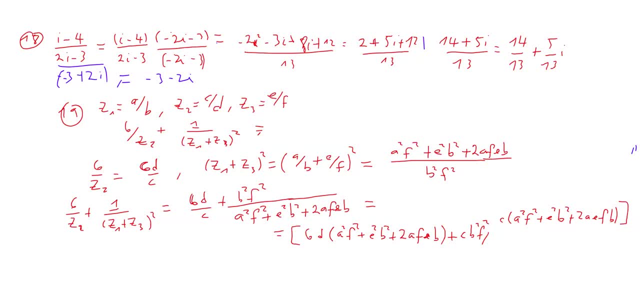 And it is equal to 14.. So it is equal to 14 plus 5 i over 13.. And now we have the real part and then the imaginary part given Then the final one was to write to demonstrate your ideas on rational number understanding. 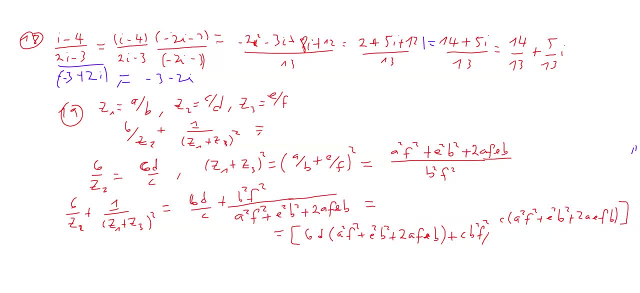 So we have z1 to be a over b, But in that sense I wrote z1 to be a comma b. I wrote z2 as well to be c comma d, And then I wrote: z3 is equal to e comma f. 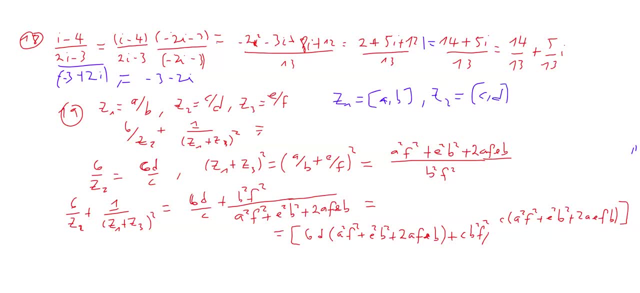 Okay, But of course we know a comma b to be the same as a over b, And then z2 is c over d, z3 is e over f, And so the question was to solve 6 over z2,. 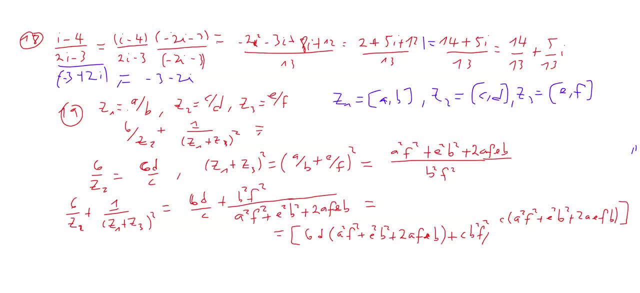 plus 1 over z1 plus z3 squared. So 6 over z2 is 6d over c, And z1 plus z3 squared was equal to a squared f squared plus e squared b squared plus 2af over b squared f squared. 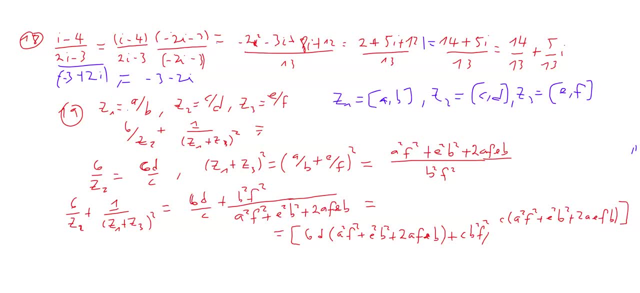 And then, if you then put it together, you'll be able to arrive at this solution here. But of course already we can write c into brackets: a squared f, squared plus e, squared b, squared plus 2af, eb, And then here we have 6d.